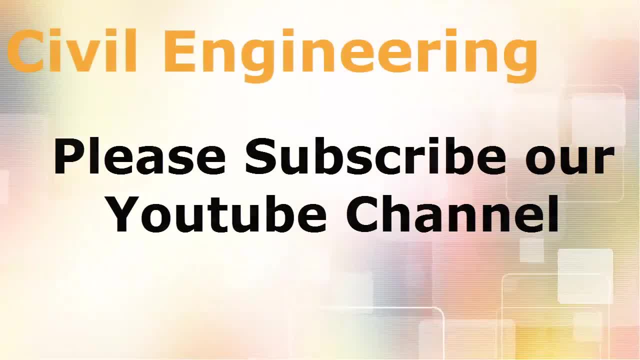 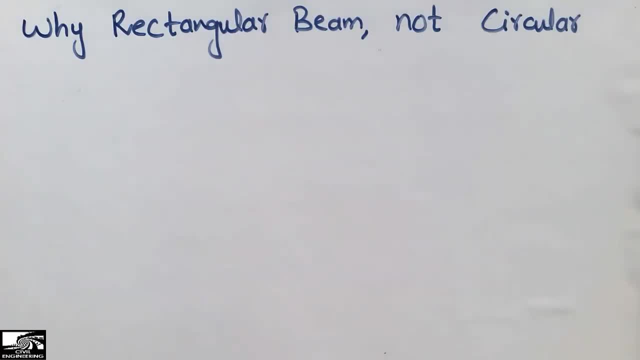 Hello guys, welcome back to the C1 Engineering YouTube channel. Please subscribe our channel for daily C1 Engineering videos. Today, our lecture is about the why we use the rectangular beam but not circular beam. However, we also use circular beams, but you may have seen very few cases in which we design the circular beam. 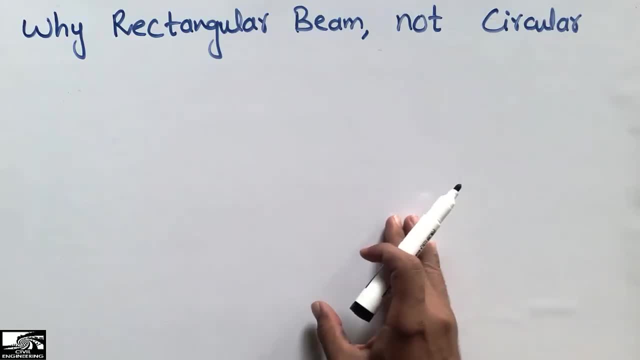 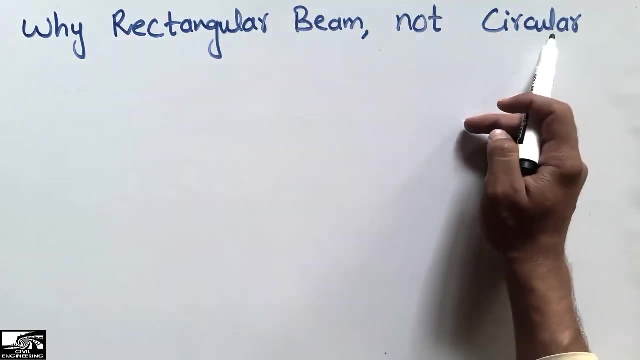 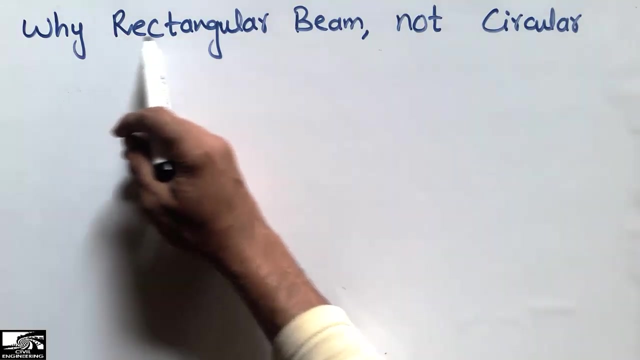 Most of the multi-story buildings or the mega projects have involved the rectangular design beams, while we don't focus on the circular beam. There are some reasons- and I will explain the two major reasons here in this video- that why we choose to design the rectangular beam for our any project and why we don't the circular beam. 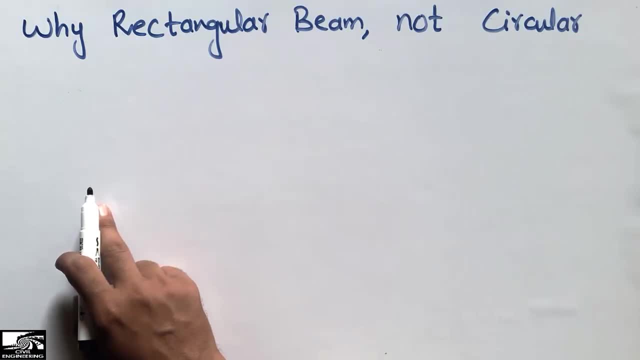 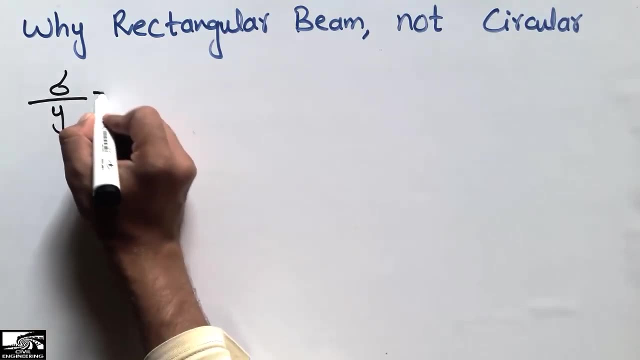 So let's first explain the first reason that why we use the rectangular beam. It's the first reason that we use the rectangular beam. It's the first reason that we use the rectangular beam, As we know that you may have seen this formula from the bending: that sigma by y is equal to the moment divided by i. 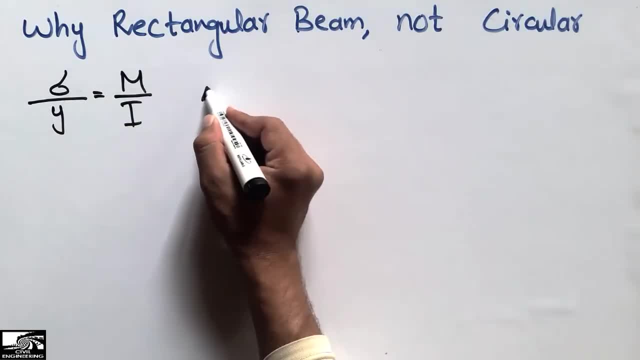 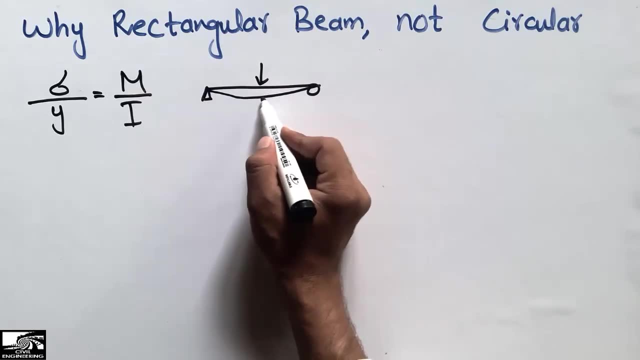 Where sigma is the bending stress. Let's consider this is in a simply supported beam. So when the load acts on this beam, so this beam is going to be deflected in this way and some bending will produce in this beam due to this load and due to this bending, bending stresses will be created in this beam. 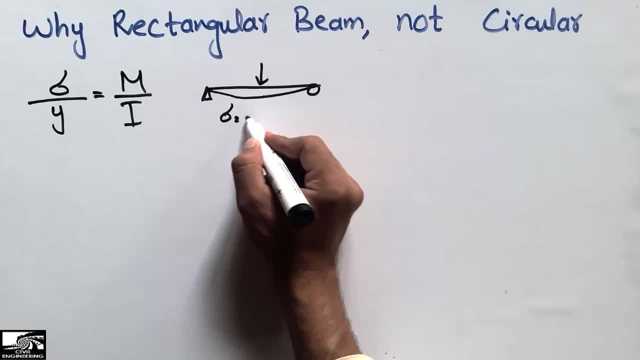 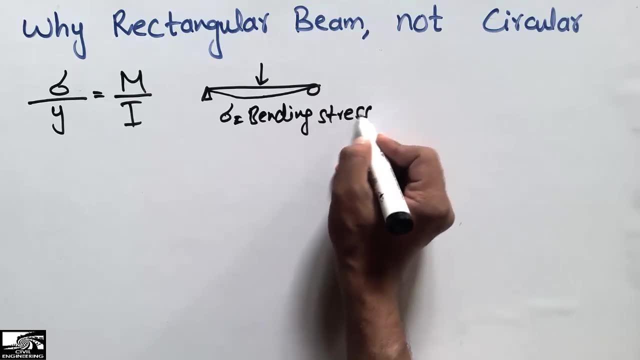 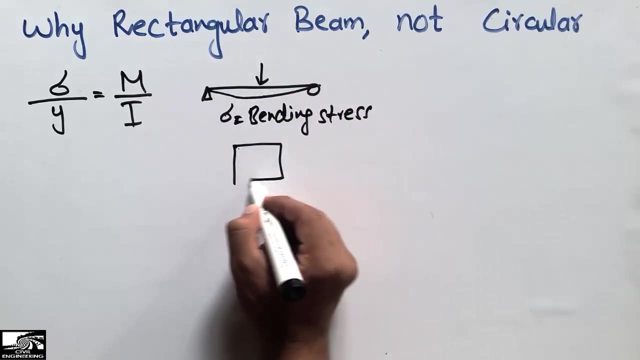 So we call sigma as the bending stresses. So the bending stress is created in this beam represented by the sigma and it is known as the bending stresses. Now why? Why, if this is my beam and this is the cross-section detail of this beam? 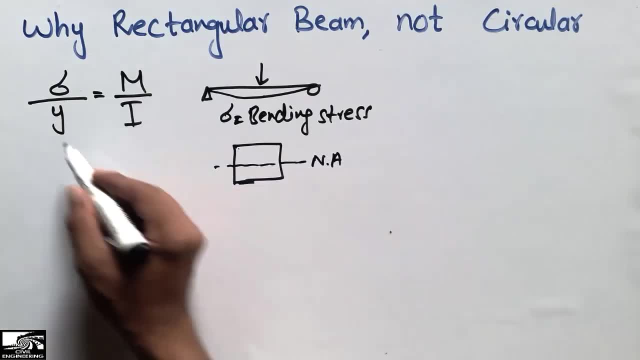 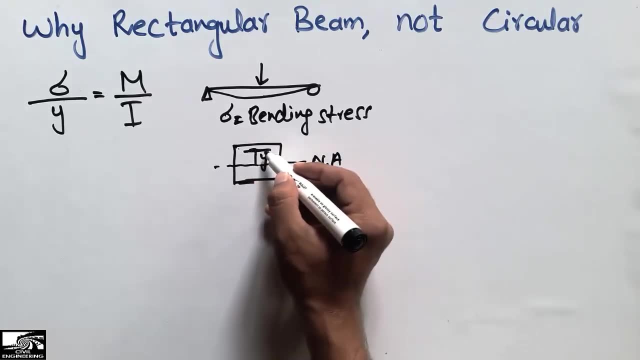 So this is the neutral axis of this beam. So y can be defined as it is the distance from the neutral axis to our point of interest. So let's suppose this is our point of interest. So this distance from the neutral axis up to this point is known as the y. 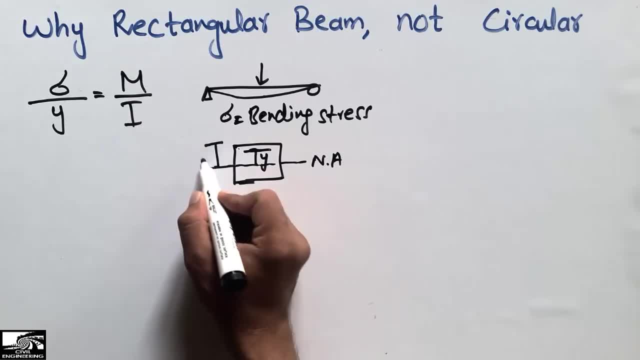 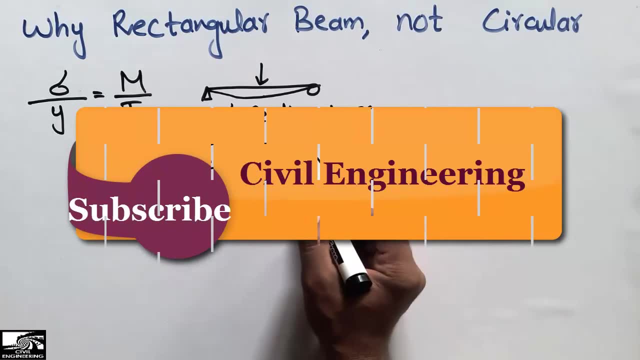 And why? Because y may be from the neutral axis up to the top of the beam. So we call this is the y. It depends on your point, where you want to find the stresses. So let's suppose from the neutral axis the distance is. my interest is this: 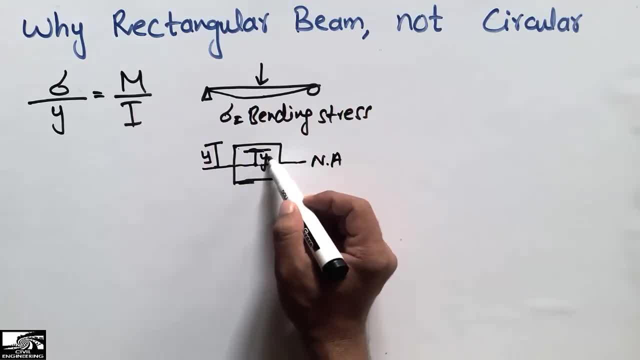 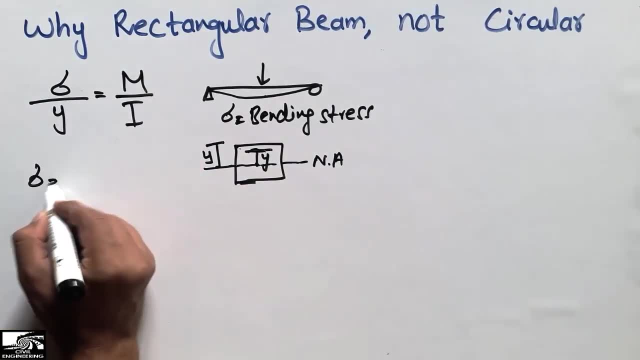 So the distance from the neutral axis up to this point is known as the y, Where m is the bending moment and i is the moment of inertia. So we can simplify this equation is like in this way: Why I place the y here, Just dividing by the i. 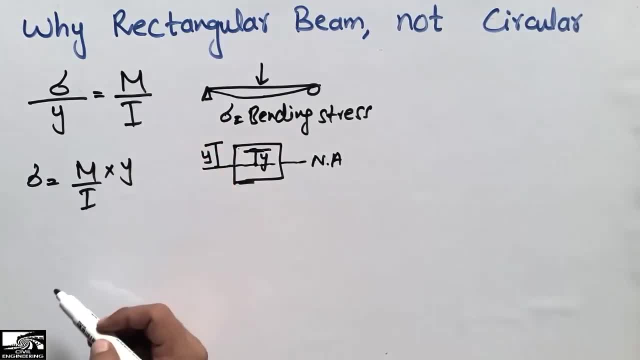 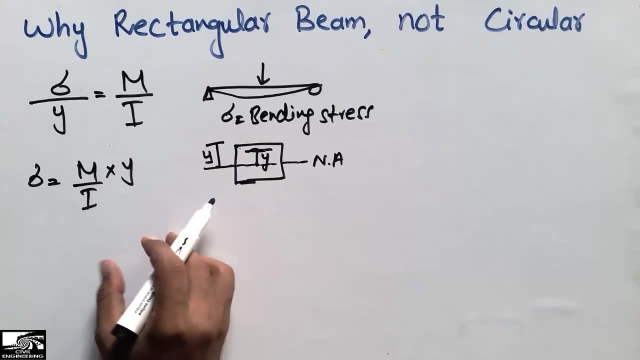 So I just put the y here into this right hand side of the equation. So now the stress is equal to the m by i into y. Now if I put my moment and y is constant, for example, for any beam, The y point is my constant and bending moment is also constant for any beam. 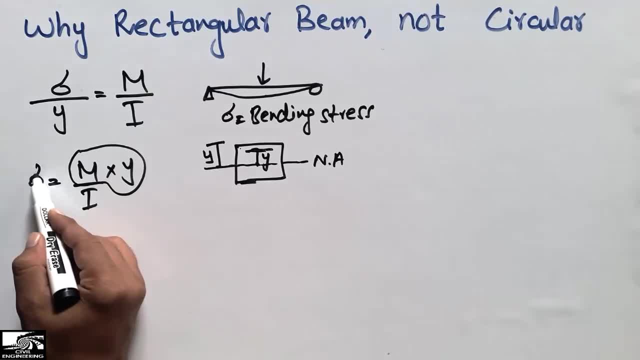 So what happens? The bending stress is in worse relation with the moment of inertia. You can see here that it is in worse relation with the moment of inertia. It means the higher the moment of inertia it is higher. so your bending stress will be lower because it is in worse relation. 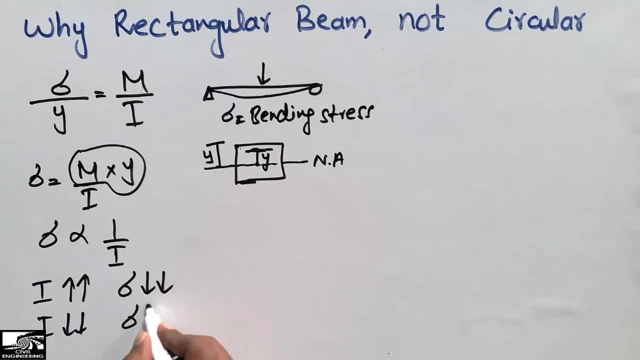 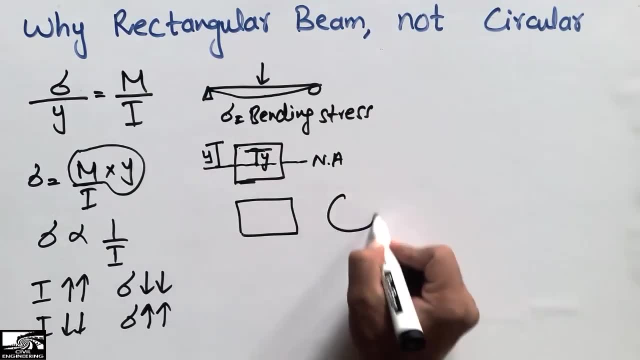 If my moment of inertia is lower, so my bending stress will be higher. So in case of the rectangular, if you have the rectangular beam and circular beam, both the beams have the same cross sectional area. Both beams have same cross sectional area, Both of the same area. so we found out that the rectangular beam has the more moment of 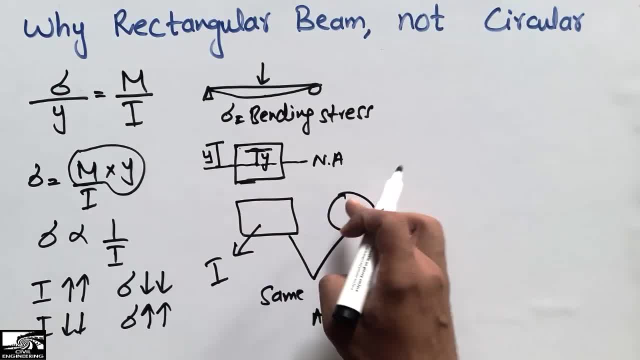 inertia and the circular beam have not more inertia as compared to the rectangular beam, While the rectangular beam has the more moment of inertia than the circular beam, while having the same cross sectional area. So we prefer to use the rectangular beam because having more moment of inertia, what happens? 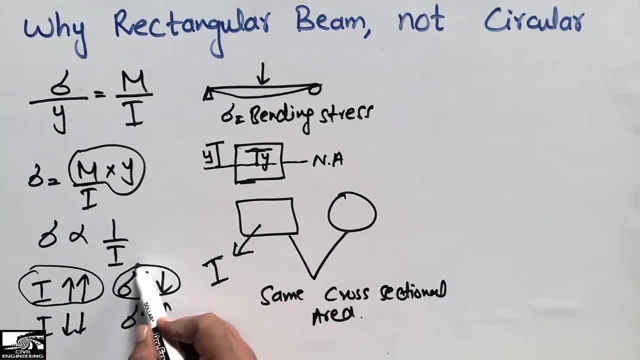 More moment of inertia, we will have the less bending stresses in our beam And we will require the less reinforcement to be used in the rectangular beam. So it will be our economical design to use the rectangular beam. That's the main reason that why we design the rectangular beam. 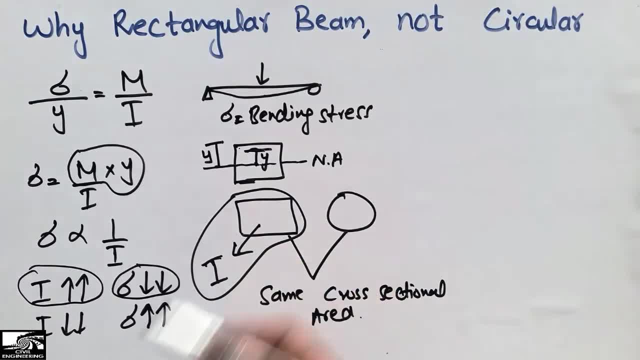 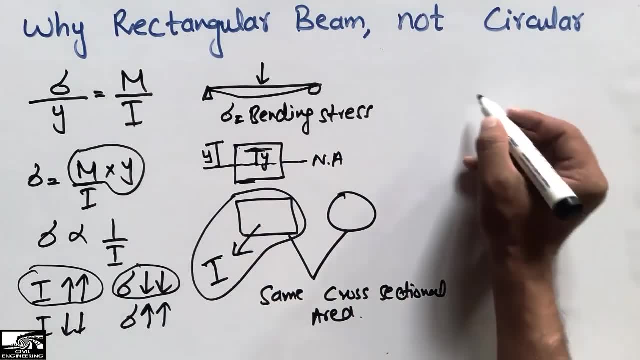 Hope you guys understand the first reason, that why we use the rectangular beam, Due to its high moment of inertia, due to its low bending, stress creates in the beam. The second reason is that- consider this is my beam. I place the beam on the side. the third: 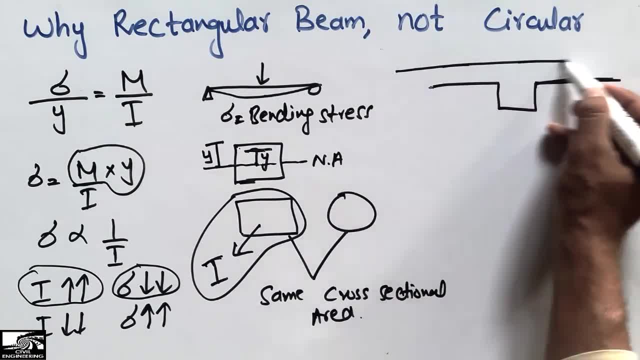 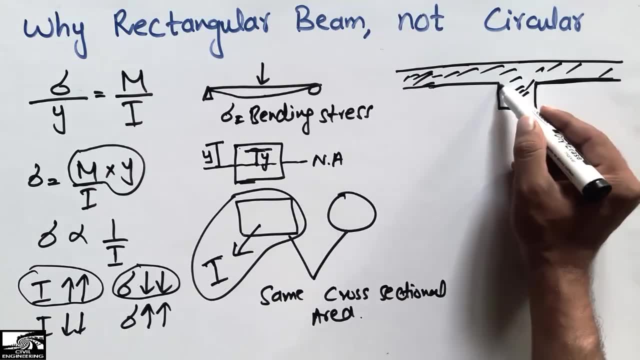 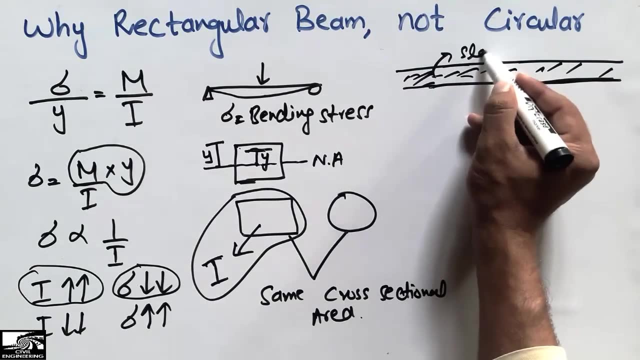 floor or the second floor of my building, And I also put the concrete in the slab and beam. So you can see this T-shape. or we can say: this is the rectangular beam, right, This is the rectangular beam we design and we put the concrete. this is my slab of 8 inches.